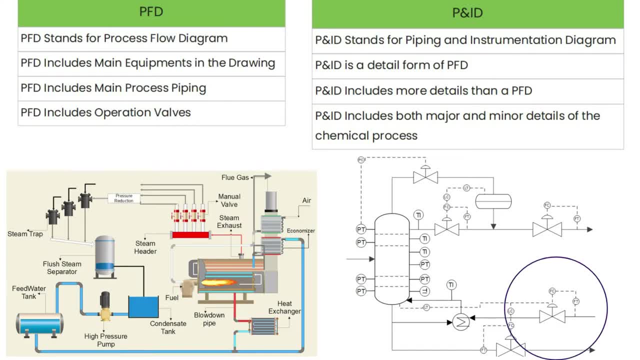 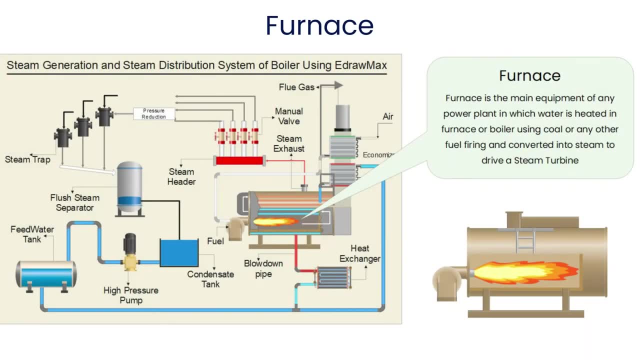 valves In the PID control loops are also defined. Let's move on PFD and understand some PFD equipments. Furnace is the main equipment of any power plant in which water is heated in furnace or boiler using coal or any other fuel firing and converted into steam to drive a steam turbine. 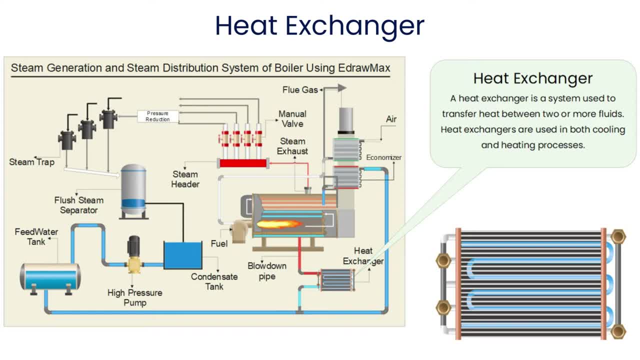 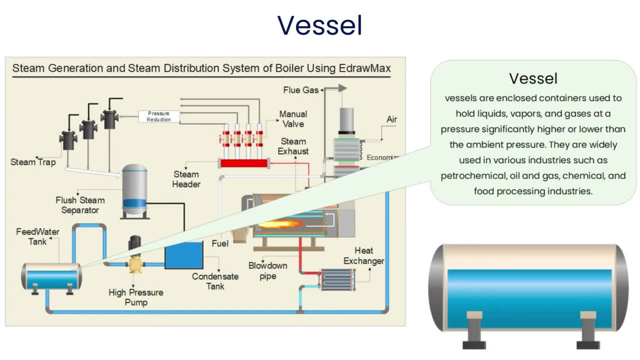 Heat exchanger is a system used to transfer heat between two or more fluids. Heat exchanger are used in both cooling and heating processes. Pills are enclosed containers used to hold liquids, vapors and gases at a pressure significantly higher or lower than the ambient pressure. These are widely used in various 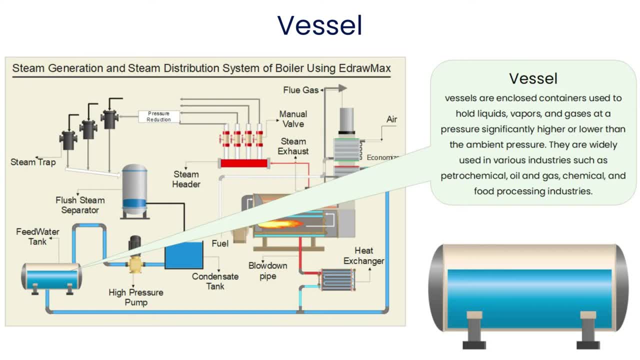 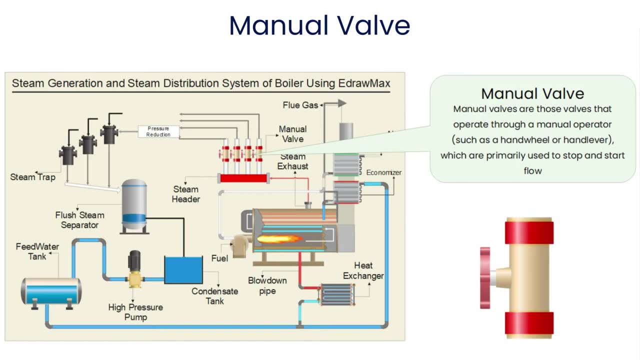 industries such as petrochemical, oil and gas, chemical and food processing industries. Manual valve are those valves that operate through a manual operator, which are primarily used to stop and start flow. An industrial pump is typically a heavy duty process pump. 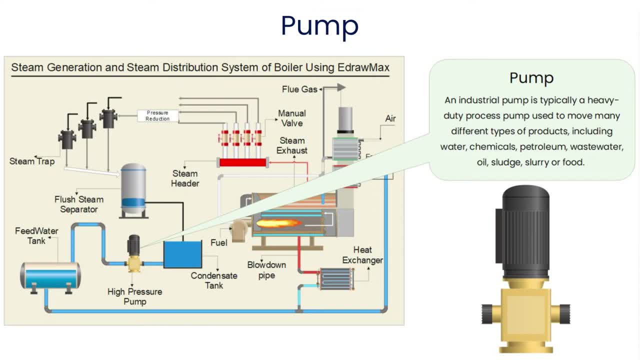 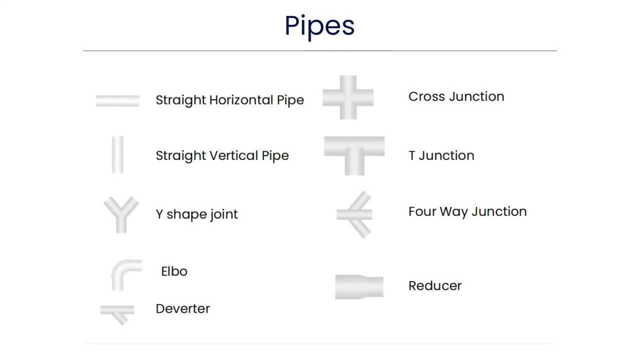 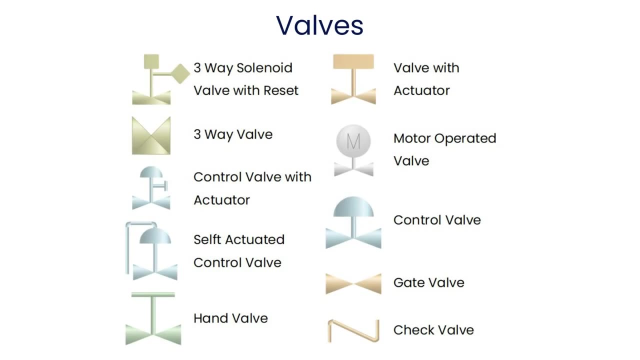 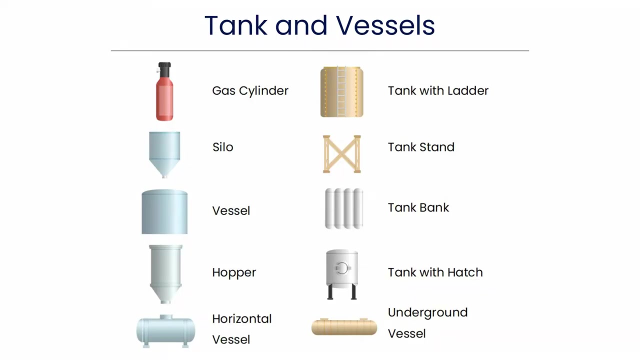 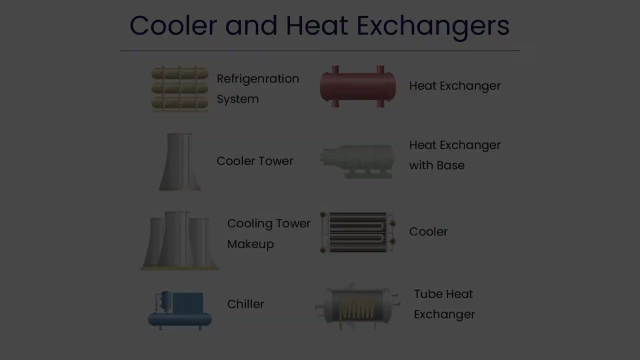 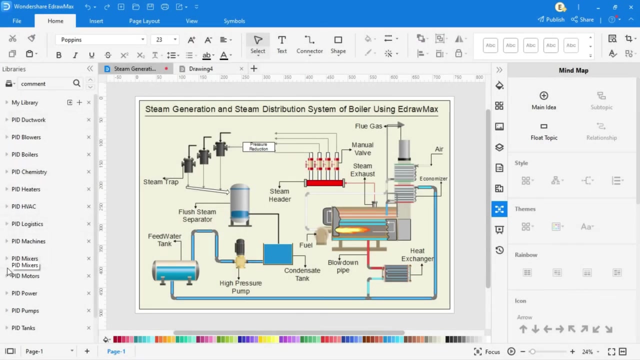 used to move many different types of products including water, chemicals, petroleum, wastewater, oil, sludge and slurry products. These are some another symbols which are commonly using in the PFD diagram. You can find all kind of PFD symbols in the eDraw MAX symbol library. 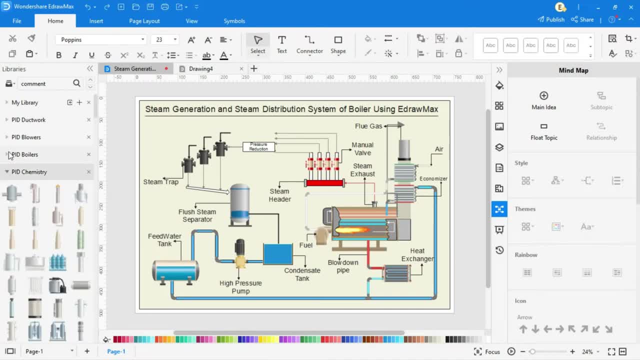 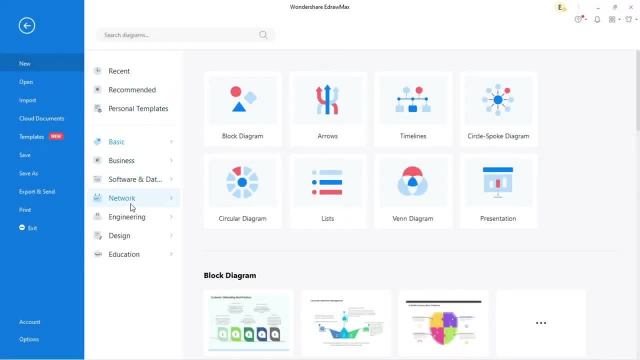 To create a new PFD drawing, go to new select engineering and then industrial engineering and create a new drawing. To create a new PFD drawing, go to new select engineering and then industrial engineering and create a new drawing. 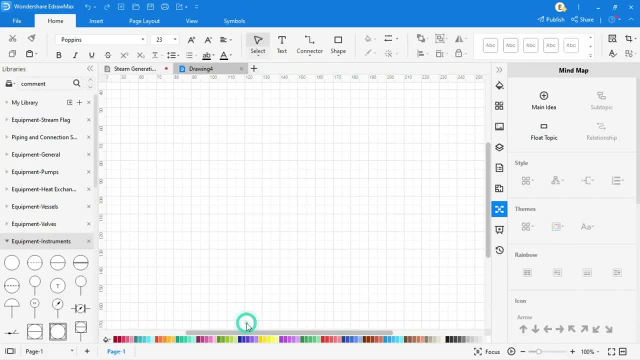 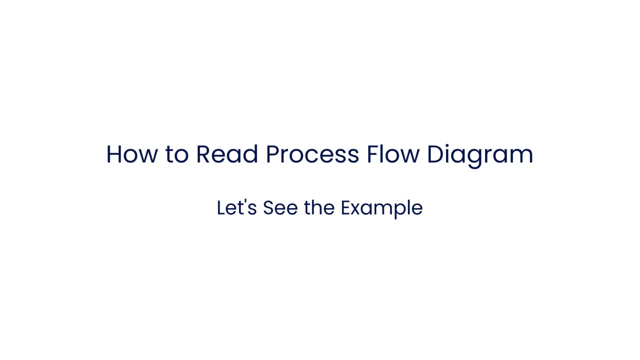 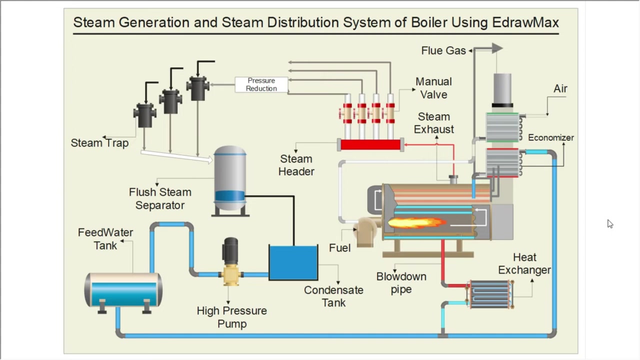 You can draw a new PFD drawing here. Let's understand how to read a process flow diagram. We can read any kind of PFD like this, But before read any PFD diagram we have need to take basic knowledge of that system in. 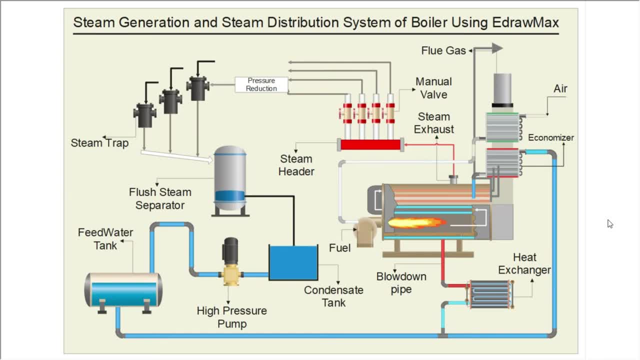 which we are going to read their PFD. You can get this knowledge from Plant Pocket Manual. Take an example of steam generation and steam distribution system of boiler PFD. In this PFD, these are main equipments. this is the furnace or boiler where water is converted. 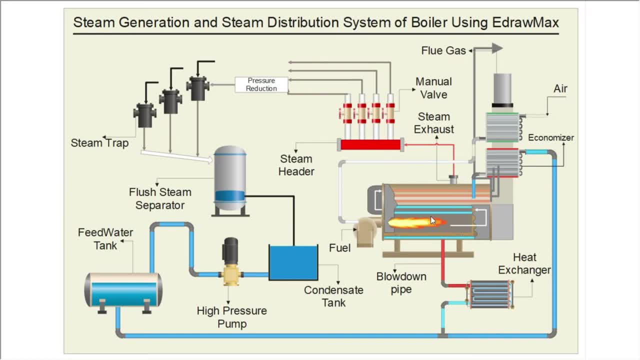 into steam. You can see that a fan symbols is also available. It means a fan is installed to supply air in the furnace for providing oxygen which helps for firing. We can track its piping is coming from heat exchanger which is available in the economizer. 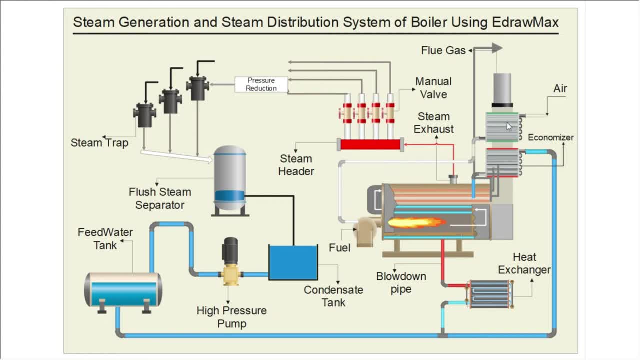 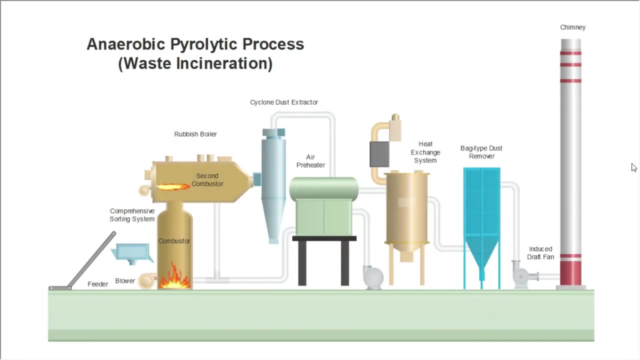 Ok, This is the economizer. From economizer, heat and fuel gases are sent to atmosphere, But some heat are taken by these heat exchanger to heat air and water. Take another example of anaerobic pyrolytic process. You can see that a firing symbols is given inside a closed vessel. 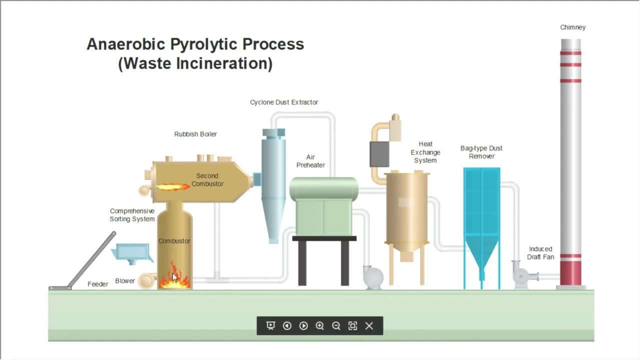 It means it is the equipment of heat generation called furnace or combustor. This is the blower symbol. It means combustor needs air supply for better firing because fire is possible due to oxygen. So this blower help to provide air supply. 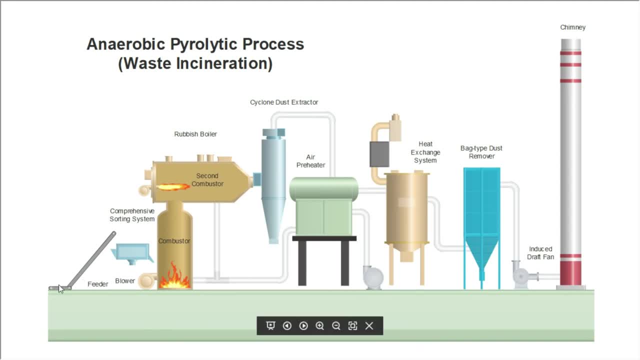 And these system is for feeding fuel supply. You can see belt or feeder. This, by default, is the main heating system in the engine, But this is left and this is the one that is used for heating, So now you do not have to do that. 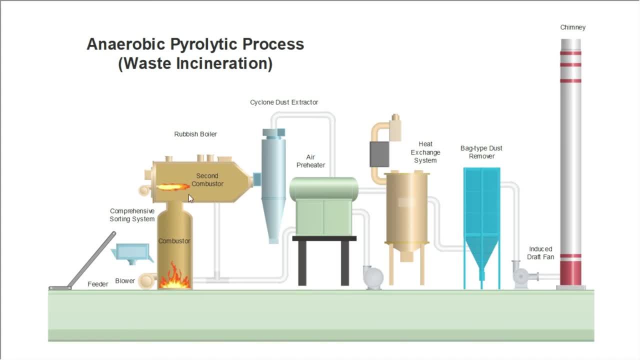 So let us go to next equipment. This is the second combustion. It is also furnace. We can clearly see that first combustion heat is coming in the second and here again firing symbol are given. It means there is need to generate more heat, Which is going to next equipment, that is, cyclone dust extractor. 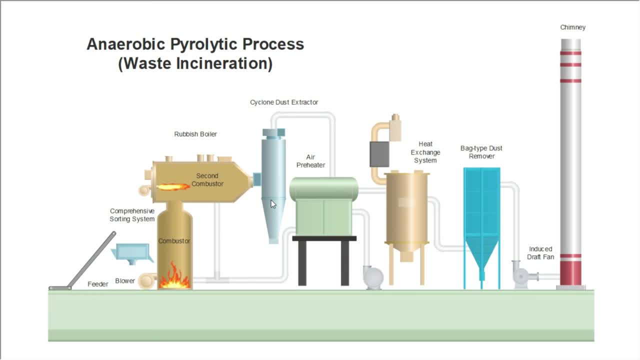 Cyclone dust extractor is used to extract dust particle which are coming from combustion. Now let us go to the next equipment, which is cyclone dust extractor. This is cyclone dust extractor. This is cyclone dust extractor buster. So like this, we can read full process flow of any kind of process industry. 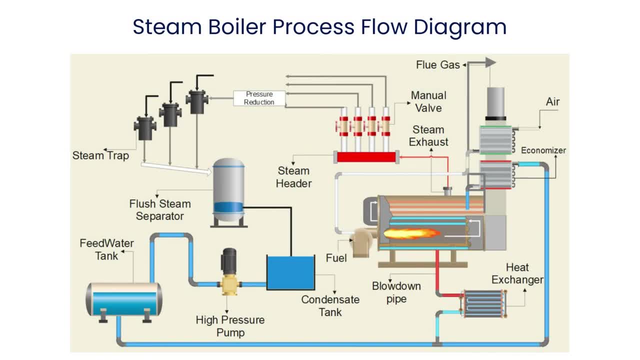 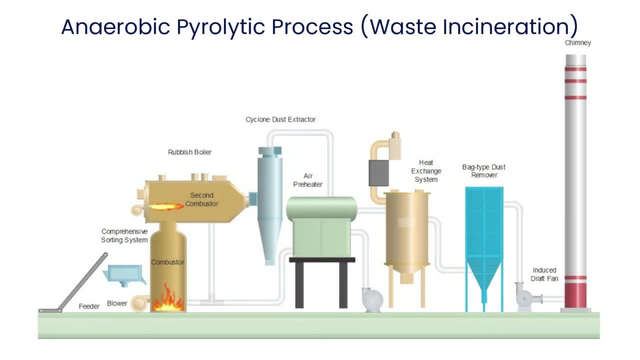 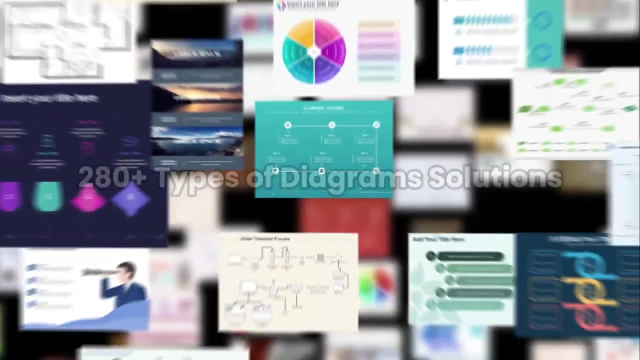 Let's see some PFD examples. This is the steam boiler PFD diagram. This is the coal power plant PFD diagram. This is the anaerobic pyrolytic process PFD diagram. And this is the air conditioning system PFD diagram. To explore more this type of videos, subscribe our channel. Thanks for watching.